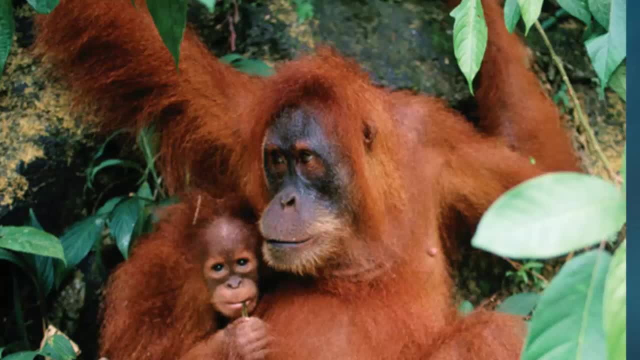 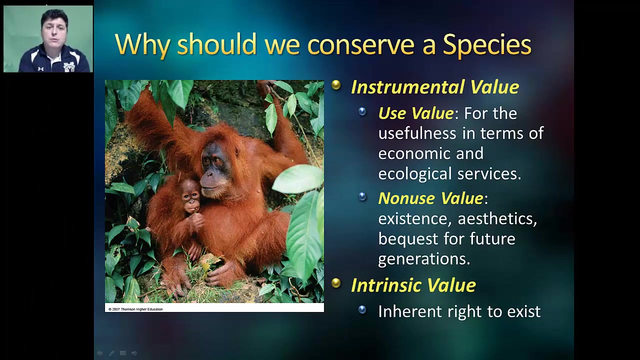 they're disappearing at a rate of about 2,000 per year due to illegal smuggling and the clearing of their forest habitat in Indonesia and Malaysia to make way for oil palm plantations. Why should we conserve a species like the orangutan? There are two reasons why conservation should be at the forefront of our minds, and that 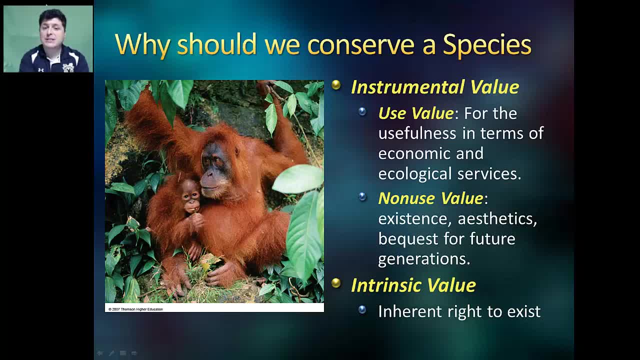 is an organism's instrumental value and its intrinsic value. An organism's instrumental value can be broken up into two parts: Its use value and its non-use value. An organism's use value is the usefulness that an organism has in terms of its economic and ecological services that it performs. 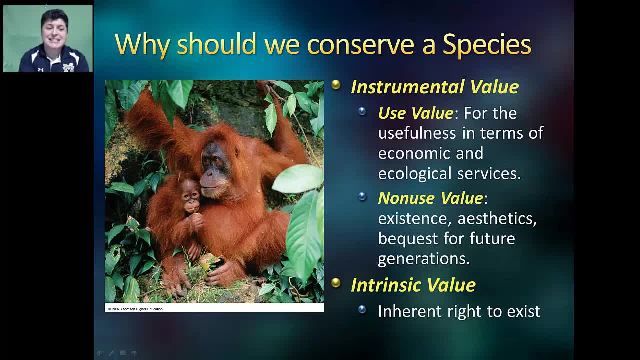 Its non-use value are its existence, aesthetic and bequest values. An existence value is just the joy that a person gets from knowing that an organism exists in the wild. Its aesthetic value is the value of an organism's value. Its non-use value is the joy that we get as we observe that organism in the wild. 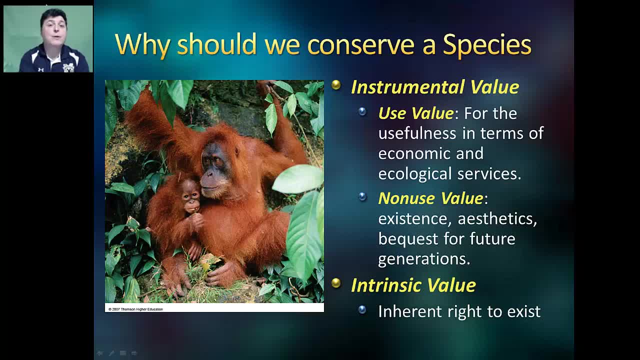 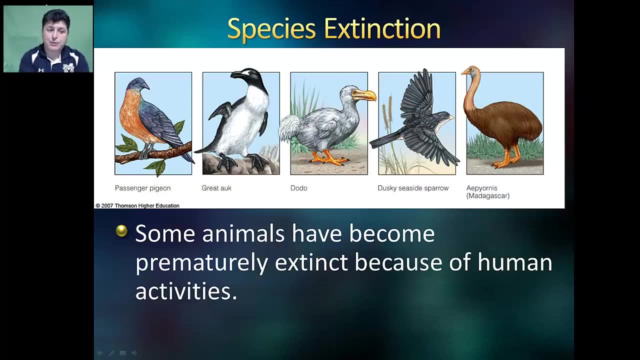 And its bequest value is the joy that we have knowing that it will be present for future generations. The intrinsic value of an organism is just its inherent right to exist Now. unfortunately, some animals have become prematurely extinct as a result of human activities, like the passenger pigeon or the dusky seaside sparrow. 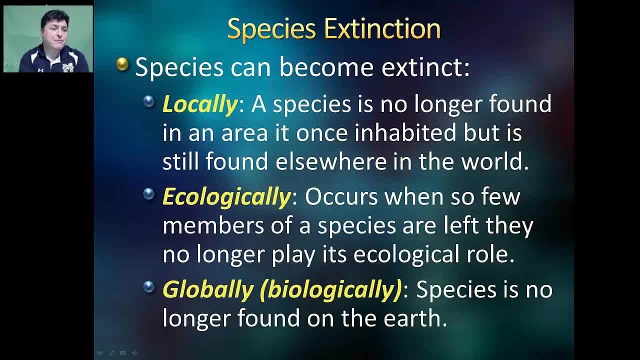 Species can go extinct in a number of different ways. They can become locally extinct, which means that it's no longer found in an area that it once inhabited, but it's still found elsewhere in the world. It can become ecologically extinct, and this occurs when there's so few members of a species. 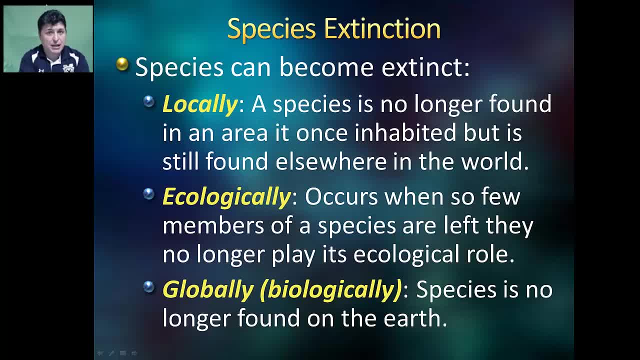 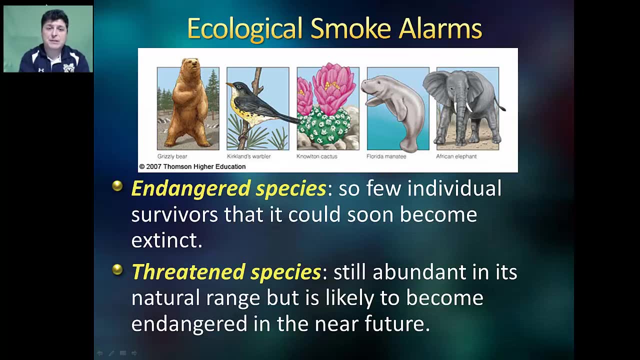 that are left, that they can no longer play its ecological role, And then, finally, organisms can become globally or biologically extinct, which means that it's no longer found on the earth. Biologists can classify species that are on their way to extinction as being either endangered, 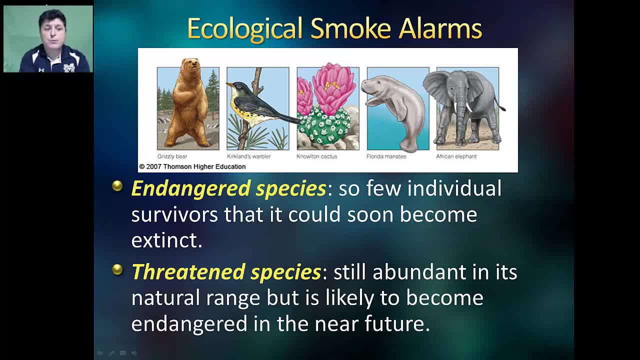 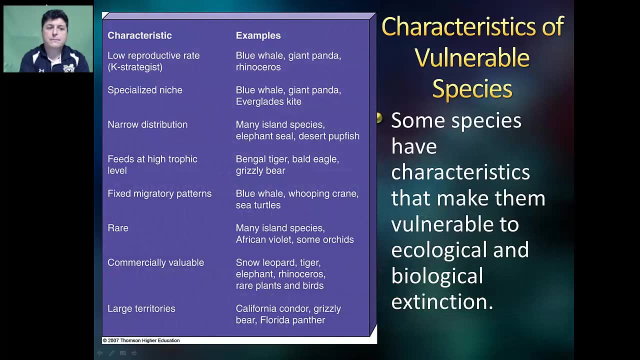 or threatened. Endangered species are those which have so few individual survivors that it could soon become extinct, Whereas threatened species are still abundant in its natural range, but it's likely to become endangered in the near future. Some species have characteristics which make them vulnerable to ecological and biological. 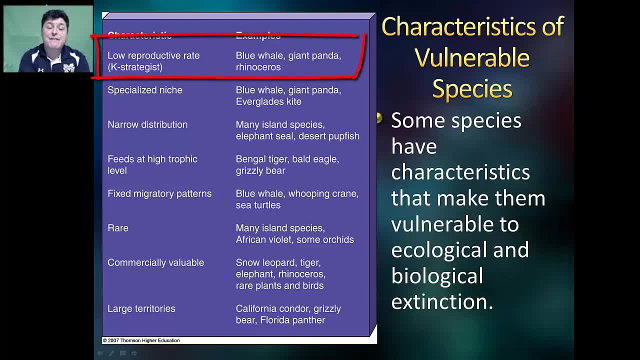 extinction. For example, they may have a very slow reproductive rate and maybe be classified as a K-selected species, like a blue whale or a giant panda. As a result of such a low reproductive rate, they'll have a really hard time recovering from a great loss. 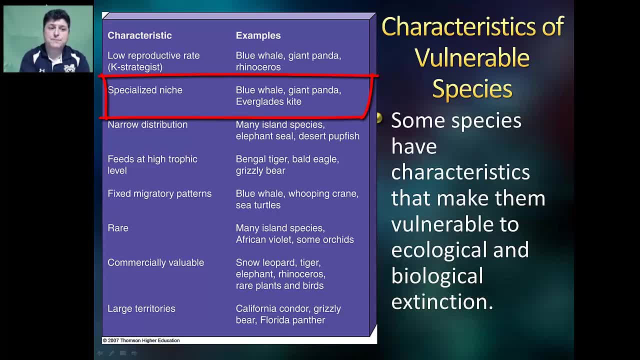 Some organisms have a very specialized niche, Like the blue whale Or the everglades Kite. When that habitat gets destroyed, that niche is no longer available for them to fill, and so therefore they would go extinct. Maybe they have a very narrow distribution or they're already rare in the environment. 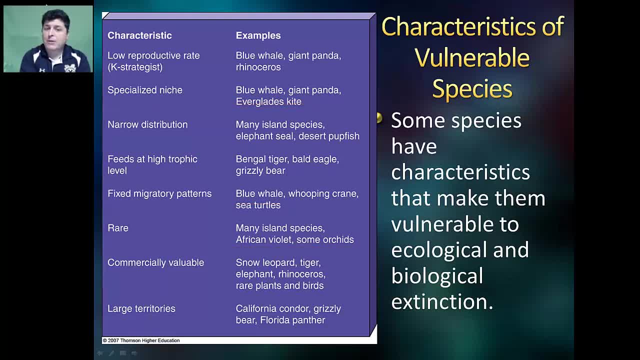 like an island species, for example, When that habitat gets destroyed or when organisms from those environments get harvested, there's so few that they will be unable to recover. Some organisms feed at high yields. Some organisms feed at low yields. Some organisms feed at high yields. 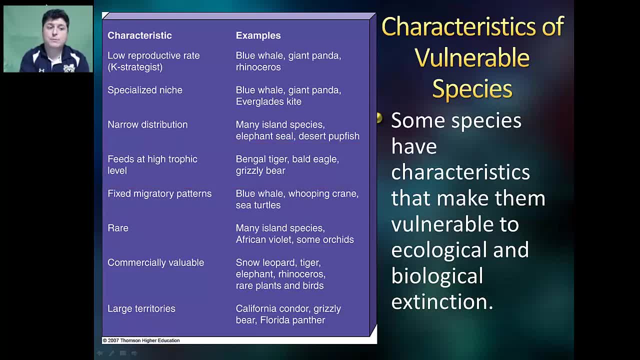 Some organisms feed at the noxious levels, like our terciary consumers, like tigers and grizzly bears, which are essential HouseButters. Not only will they die, but they will land upon a roadside tire And their habitat is devastated. their prey species will be eliminated. 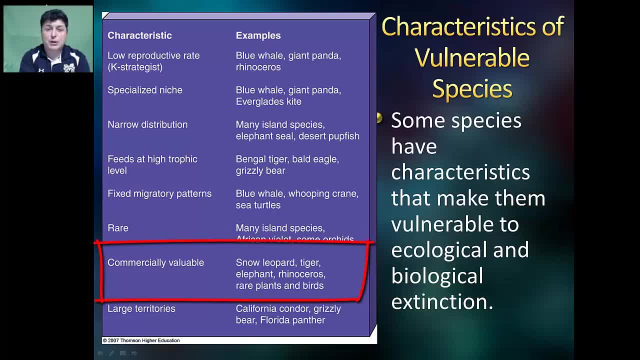 Then they will be at greater risk for extinction. Then, finally, there are some organisms that are commercially valuable as a result of their meat, fur or the presence of tusks or horns, like snow leopards or rhinoceros, and when 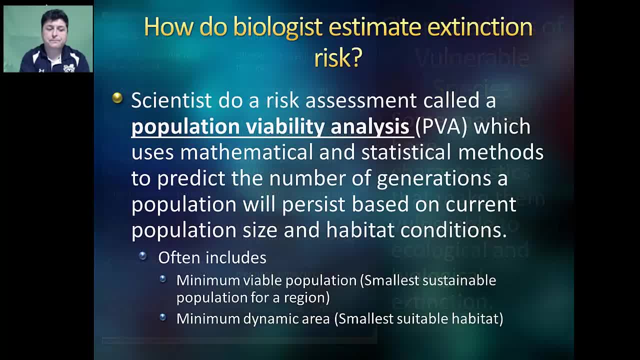 they are overharvested, they are at greater risk for extinction. So how would a biologist estimate an extinction risk? Well, scientists will do a risk assessment, called a population viability analysis, which uses mathematical and statistical methods to predict the number of generations that a population will persist. 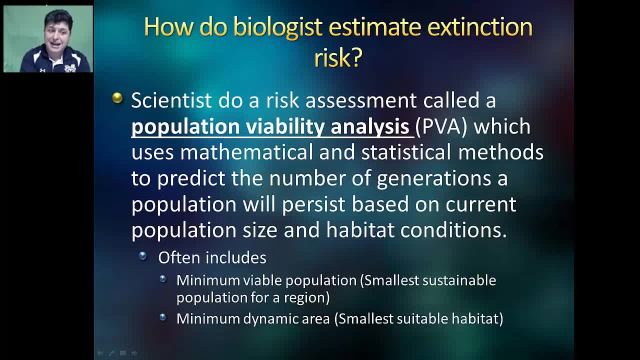 based upon its current population, size and habitat conditions. This often includes doing a minimum viable population assessment, in which we determine the smallest number of individuals which will sustain a population in a given region, as well as the minimum dynamic area analysis, where we figure out what's the smallest suitable habitat that can sustain a particular population. 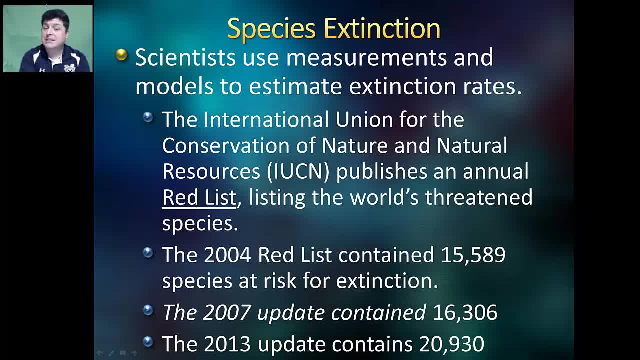 Scientists use these measurements and models to estimate extinction rates. The International Union for the Conservation of Nature and Natural Resources, the IUCN, publishes an annual red list listing the world's threatened species. In 2004,, the list contained 15,589 individuals. 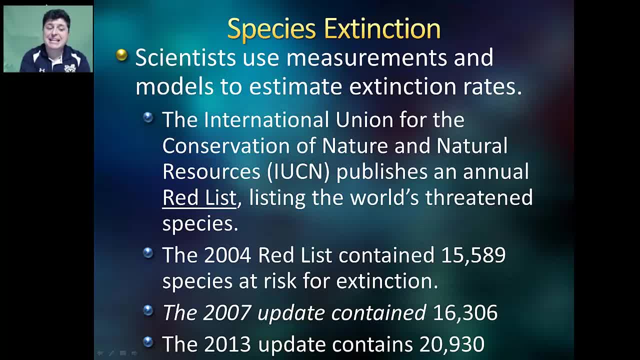 The 2007 update contained 16,306.. And most recently, the 2013 update contains 20,930 species at risk for extinction. As you can see, with each consecutive update, the number of species at risk for extinction increases. 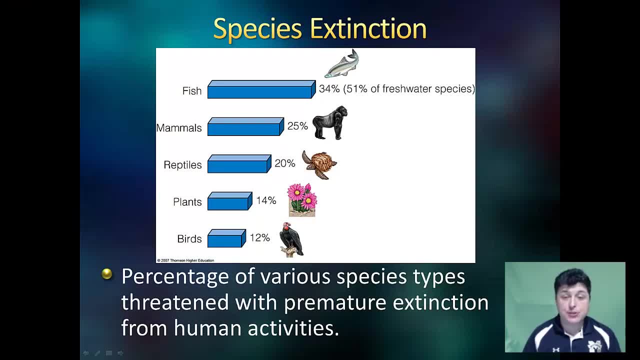 Now certain species types are at greater risk for extinction than others. There are over 34% of the world's fish species, 51% of our freshwater species that are at risk for premature extinction, 25% of all mammals, 20% of reptiles. 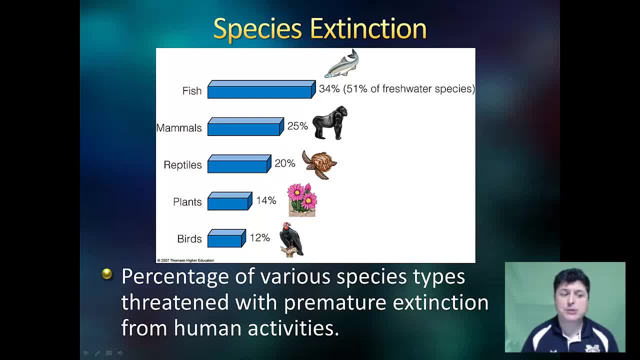 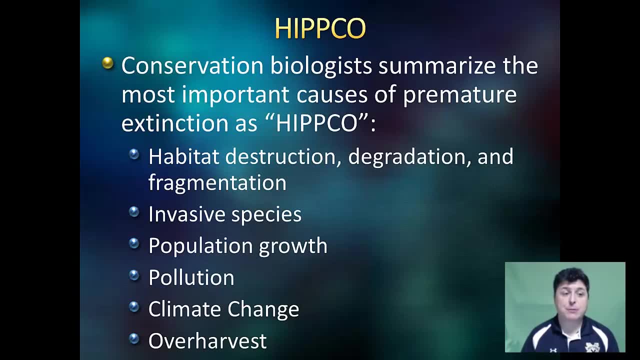 14% of plants and 12% of birds are threatened with premature extinction from human activities. Conservation biologists can summarize the most important causes of premature extinction as HIPCO. It used to just be HIPO, but we've added an additional C to include climate change. 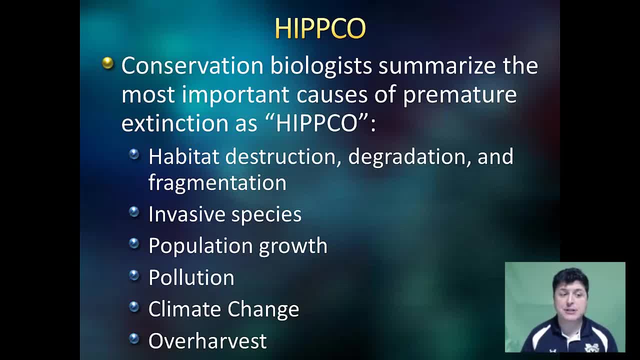 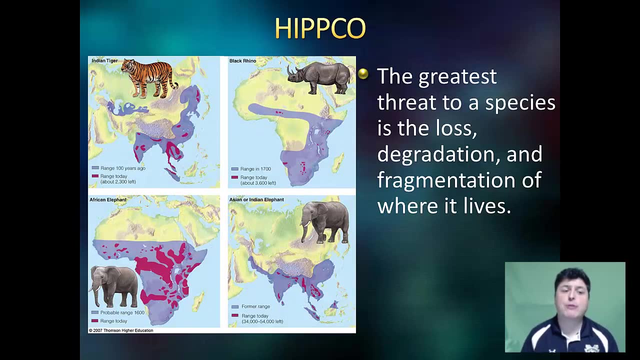 H will stand for Habitat Destruction, Degradation and Fragmentation. I stands for Invasive Species, P for Population Growth, P for Pollution and then our O for Overharvest. So scientists believe that the greatest threat to a species 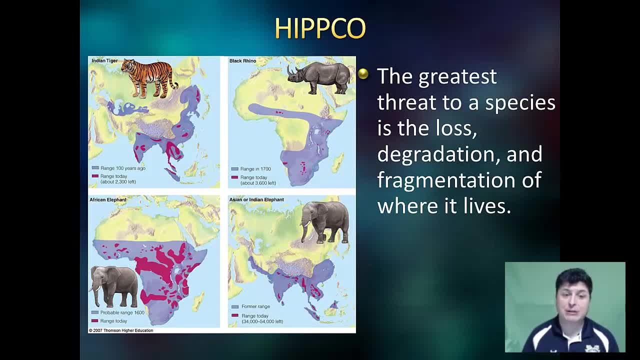 is the loss, degradation and fragmentation of where it lives. Now, certain types of species are particularly vulnerable to local and regional extinction because of habitat fragmentation. They would include species that are rare, species that need to roam unhindered over large areas. 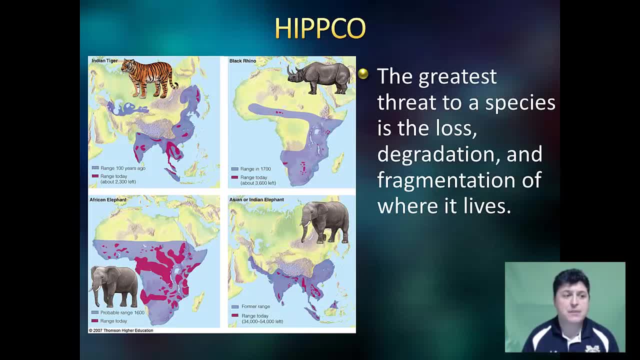 and species that have a low reproductive capacity. Here we can examine four major species- The Indian tiger, the black rhino, the African tiger, the African elephant and the Asian or Indian elephant- and compare their range from many years ago to today. 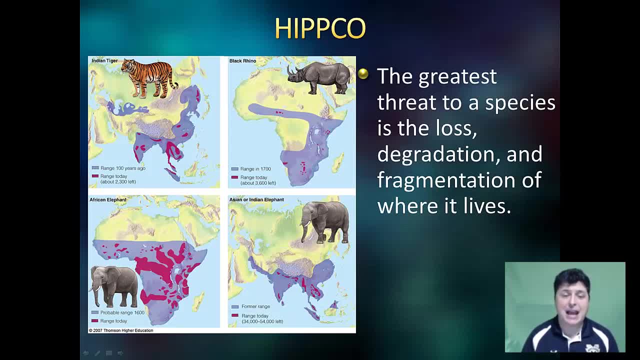 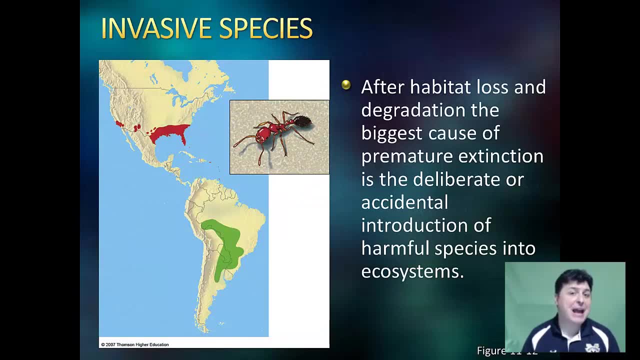 and see that, as a result of human activity and hunting, we have greatly reduced the range of these organisms. After habitat loss and degradation, the biggest cause of premature extinction is the deliberate or accidental introduction of a harmful species into an ecosystem, like the Argentinian elephant. 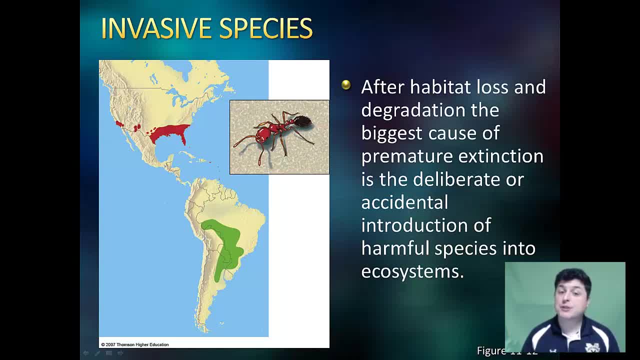 or the African ant. Most species introductions are beneficial to us, although they often displace native species. We depend heavily on introduced species for ecosystem services, food, shelter, medicine and aesthetic enjoyment. Introduced corn, wheat, rice and other food crops. 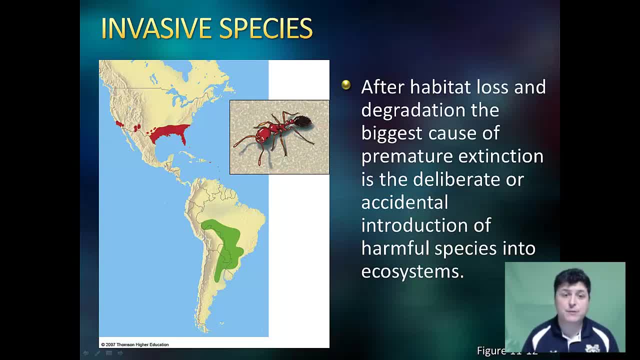 provide more than 98% of the United States' food supply. Similarly, non-native tree species are grown in 85% of the world's tree plantations. the problem is that many of the introduced species have no natural predators, competitors, parasites. 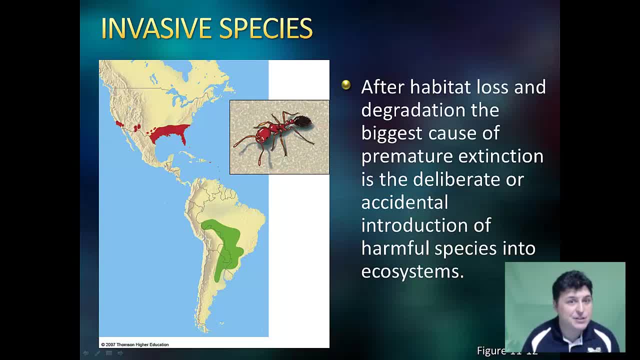 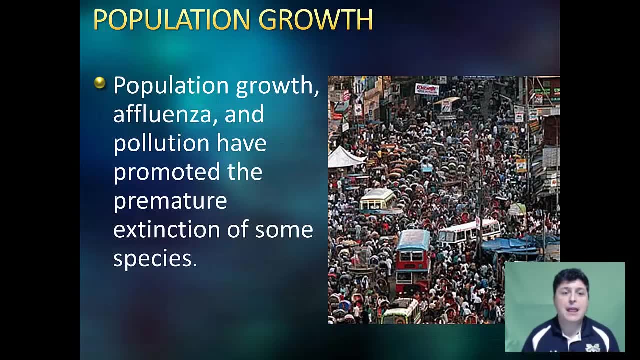 or pathogens to control their numbers. Such non-native species can wipe out populations of native ones. Human population growth and excessive and wasteful consumption of resources have greatly expanded the human ecological footprint, which has eliminated vast areas of wildlife habitat. Acting together, these factors have caused premature extinction of many species. 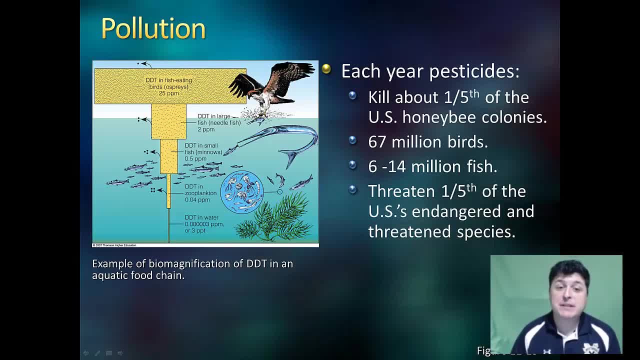 Pollution also threatens some species with extinction has been shown by the unintended effects of certain pesticides. Each year pesticides kill about one-fifth of the US honeybee colonies. They kill 67 million birds, 6 to 14 million fish. 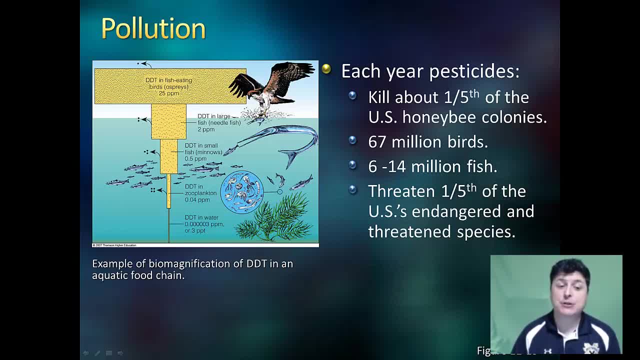 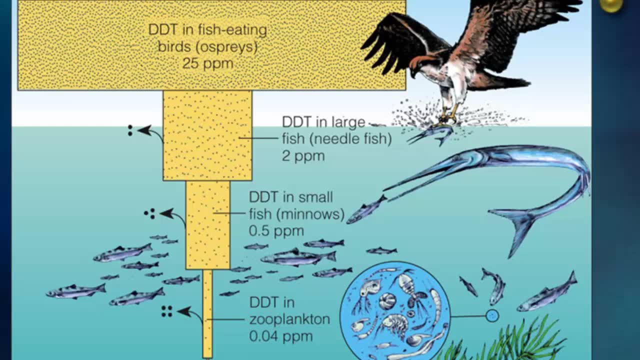 and threaten one-fifth of the US endangered and threatened species During the 19th century. during the 1950s and 1960s, populations of fish-eating birds such as ospreys, brown pelicans and bald eagles plummeted. 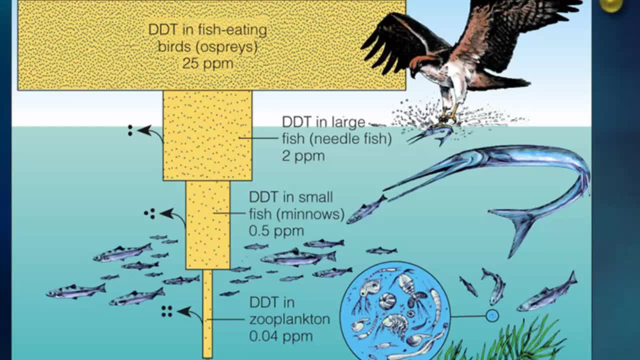 A chemical derived from pesticide DDT, when biologically magnified in food webs, made the birds' eggshells so fragile they could not reproduce successfully. Also hard hit were such predatory birds as the prairie falcon sparrowhawk and peregrine falcon. 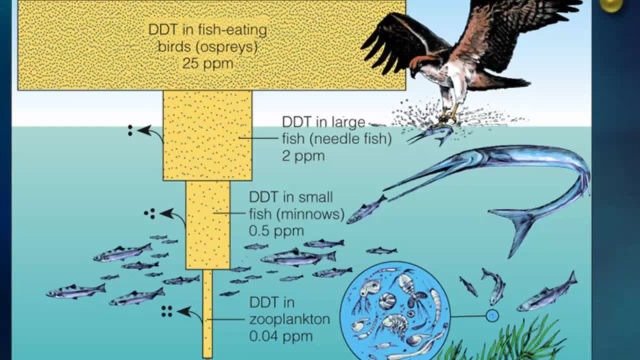 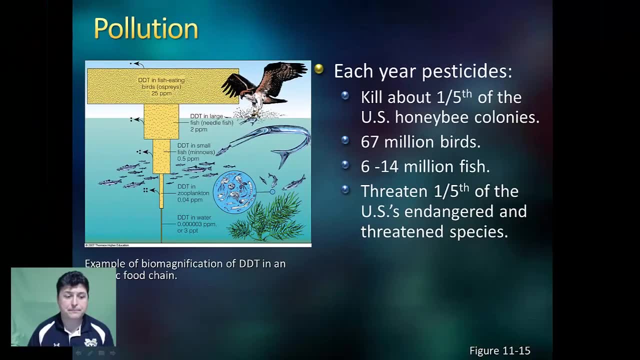 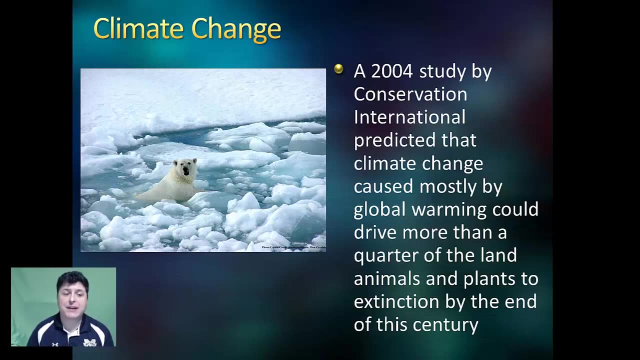 which helped to control rabbits, ground squirrels and other crop eaters. Since the US ban on DDT in 1972, most of these species have made a comeback. A 2004 study by Conservation International predicted that climate change. 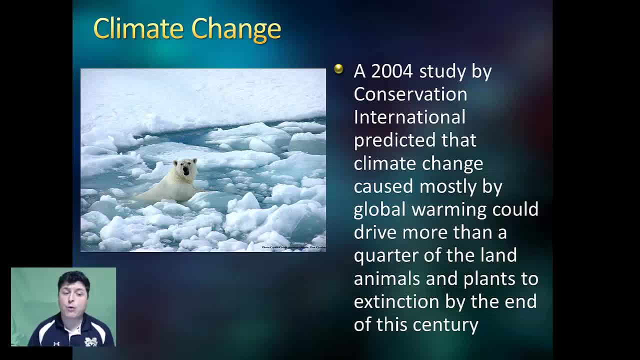 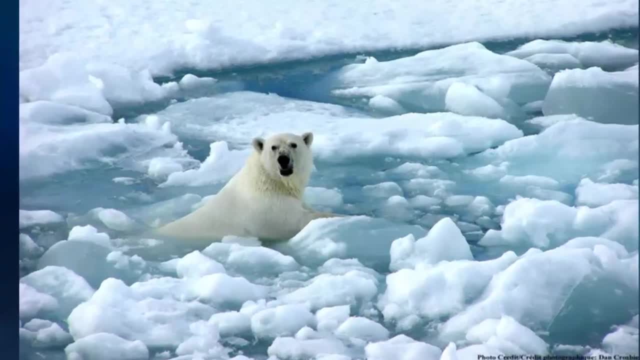 caused mostly by global warming, could drive more than one-quarter of the land, animals and plants to extinction by the end of this century. The world's 20,000 to 25,000 polar bears are at great risk. Evidence shows that the Arctic warming. 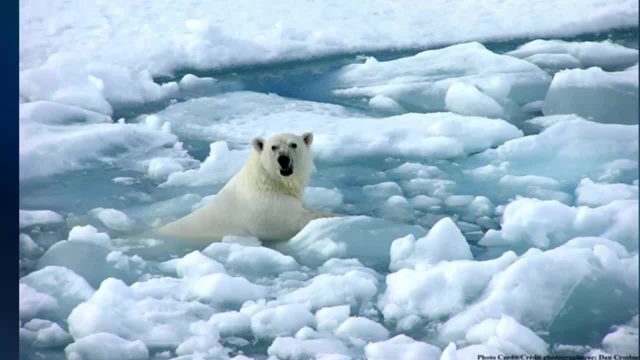 is twice as fast as the rest of the world and that the average annual area of floating summer sea ice in the Arctic is declining and breaking up earlier each year. This means that polar bears have less time to feed and to store fat they need in order to survive. 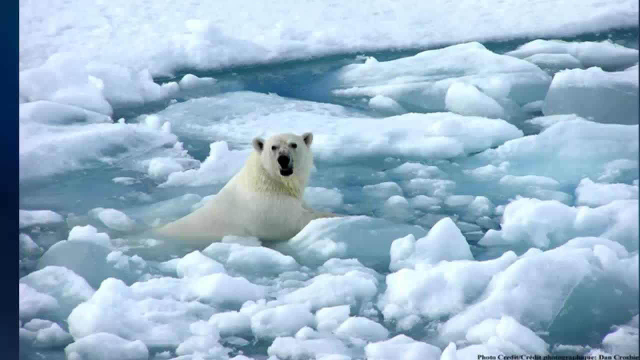 their summer and fall months of fasting. Polar bears are strong swimmers, but ice shrinkage has forced them to swim longer distances to find enough food and to spend more time during the winter hunting on land where prey is nearly impossible to find. Several studies link global warming. 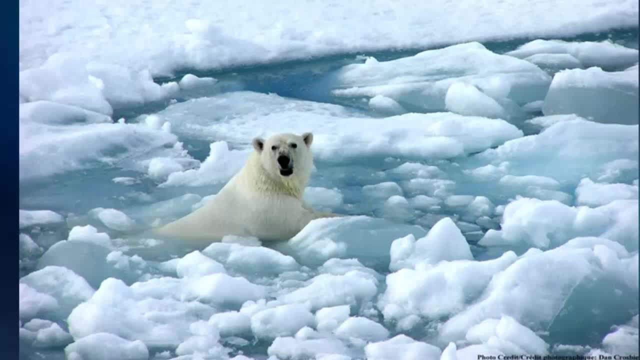 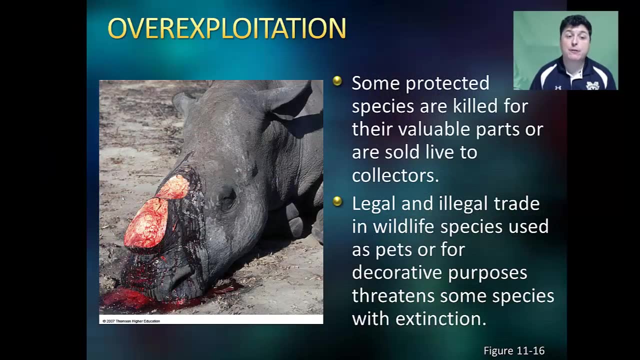 and diminished sea ice to polar bears drowning or starving while in search of prey. Some protected species are killed for their valuable parts or sold live to collectors. Legal and illegal trade in wildlife species used as pets or for decorative purposes threaten some species with extinction. 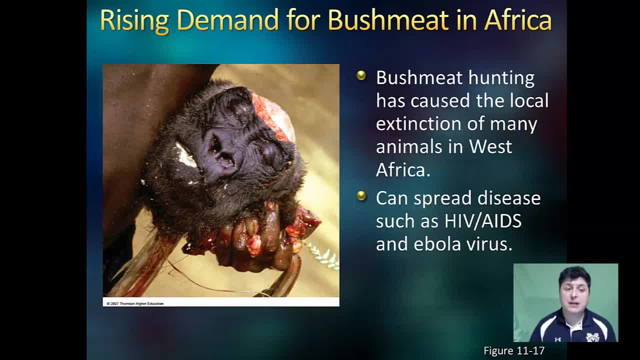 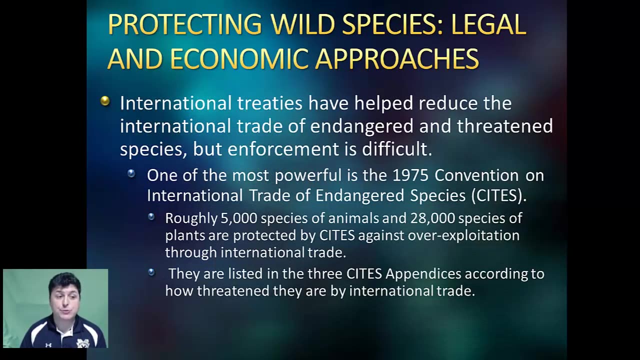 Bushmeat hunting has caused the local extinction of many animals in West Africa. The hunting for bushmeat can actually spread diseases such as HIV and the Ebola virus. International treaties have helped reduce the international trade of endangered and threatened species, but enforcement is very difficult.